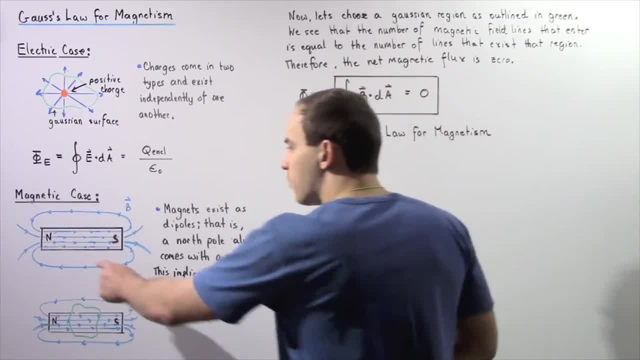 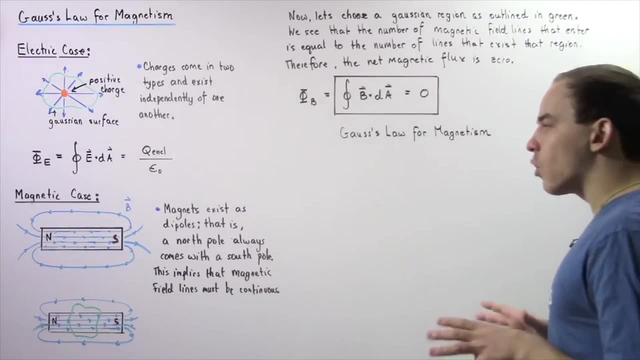 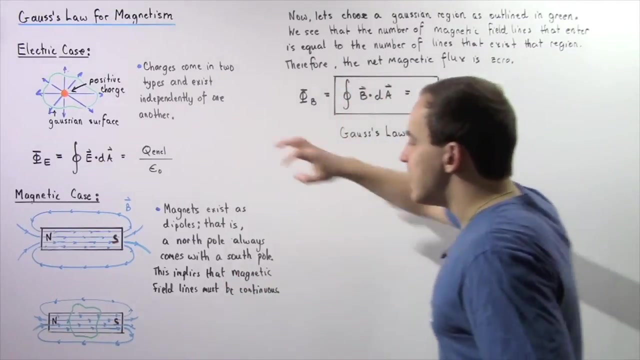 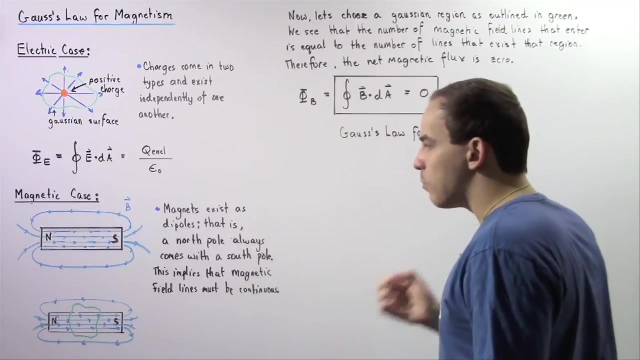 going to examine magnets. So let's suppose we have the following bar magnet. So recall that any time we have any sort of magnet, that magnet will always have a north pole and a south pole. So magnets exist as dipoles. That is, we have a north pole and a south pole, So this is our north pole. 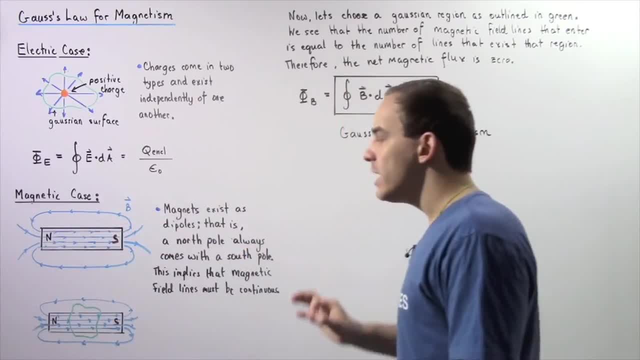 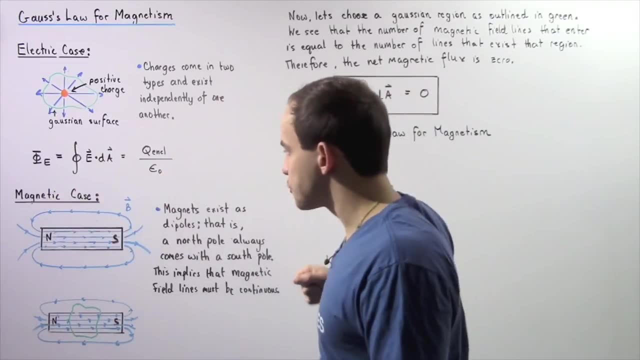 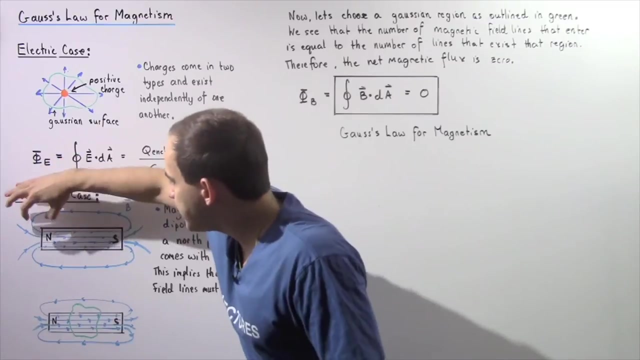 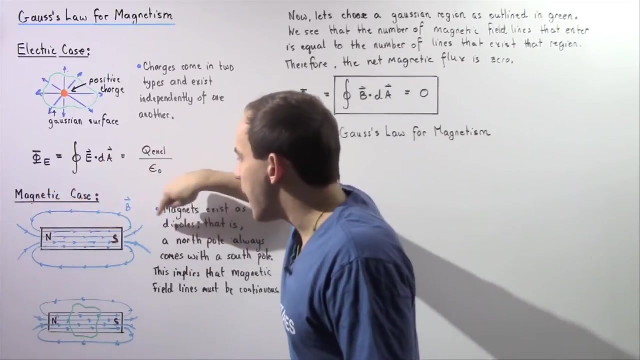 and this is our south pole. Now, if we are to draw our magnetic field lines, they will look as follows. So they will form the following loops, and these loops will essentially point, beginning at the north pole and passing through our south pole, as shown by the following regions. So this 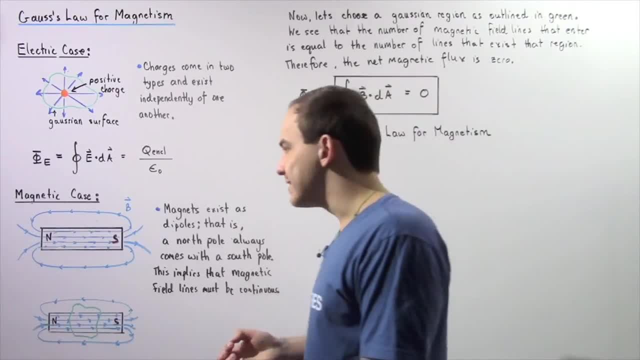 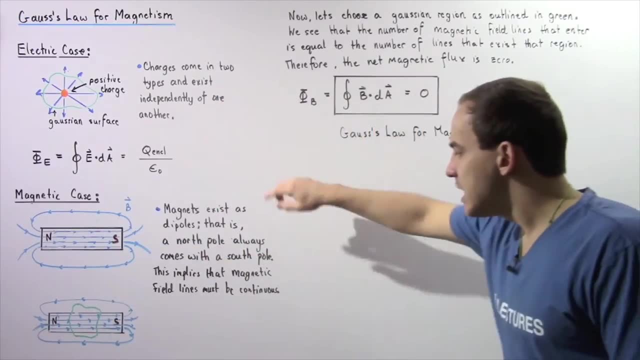 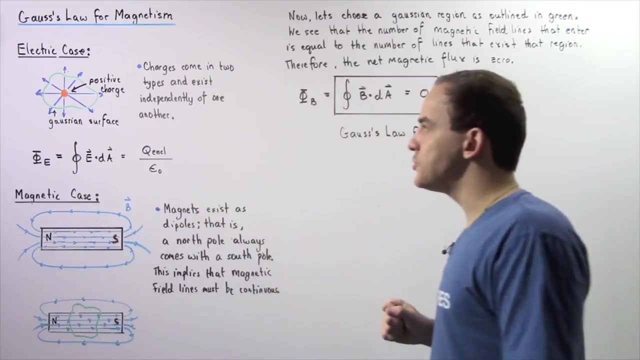 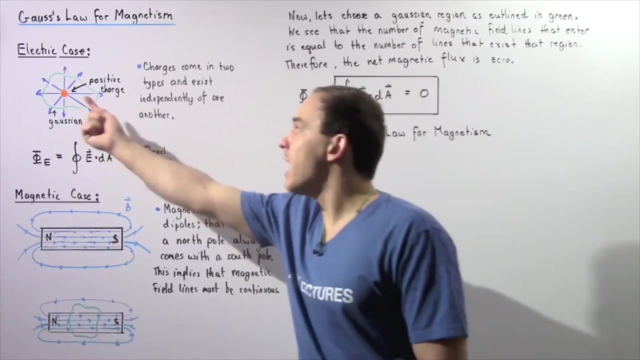 basically implies that because magnets come as dipoles, meaning we have a north pole and a south pole, this implies that magnetic field lines must be continuous, as shown in the following region. So this is a clear distinction from the electric case, Because our positive charge can exist in an isolated form. we see 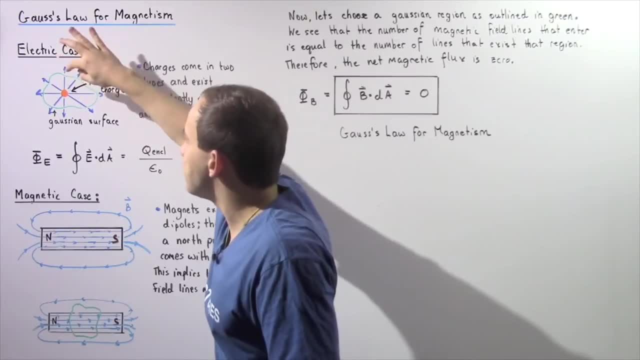 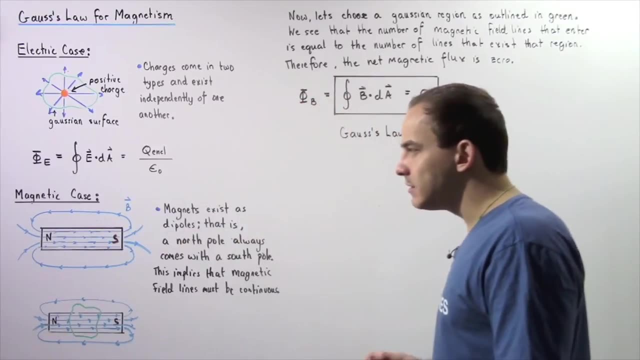 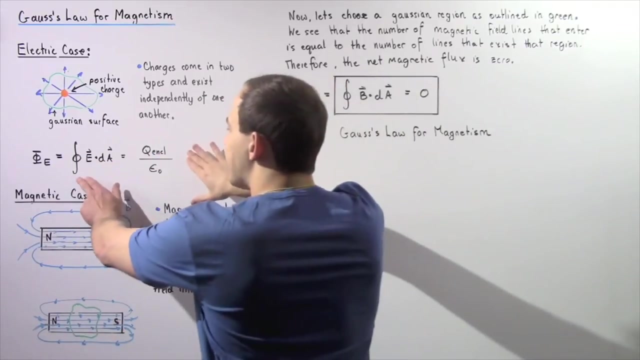 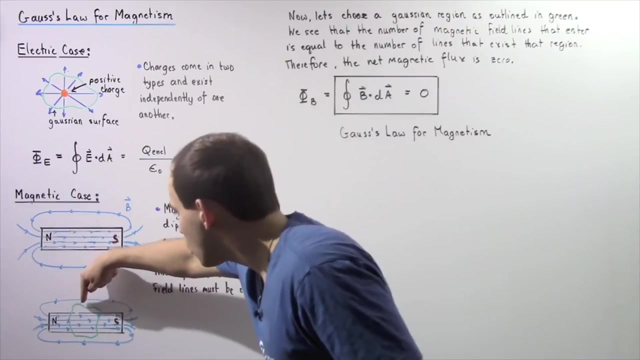 that our electric field lines begin on the positive charge and extend outward, versus in this case, where our magnetic field lines essentially form the following loops: So let's define the following analogous equation for magnetism: So let's choose a Gaussian surface. So let's choose the following Gaussian surface: 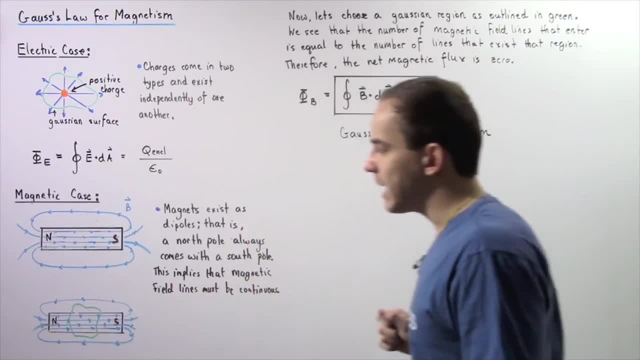 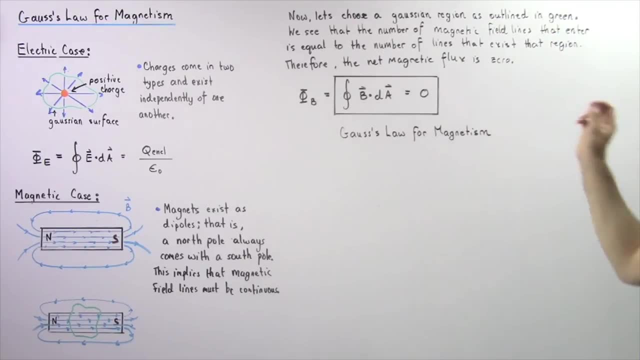 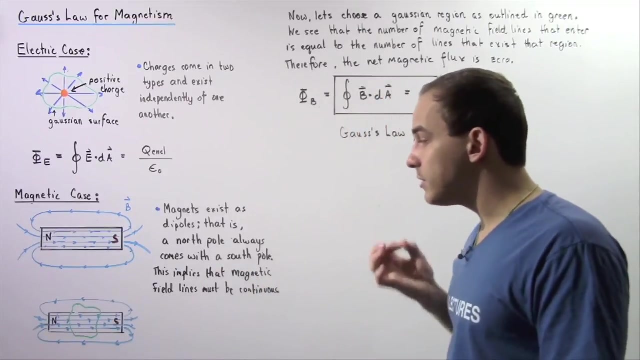 So we choose a Gaussian surface as shown by the following regions outline. So we see that the number of magnetic field lines that enter our Gaussian surface from the left side is equal to the number of magnetic field lines that exit this same region on the right side. And that implies that because the number of magnetic field lines entering is equal, 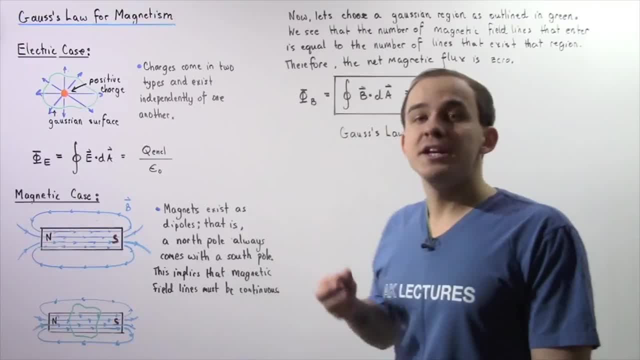 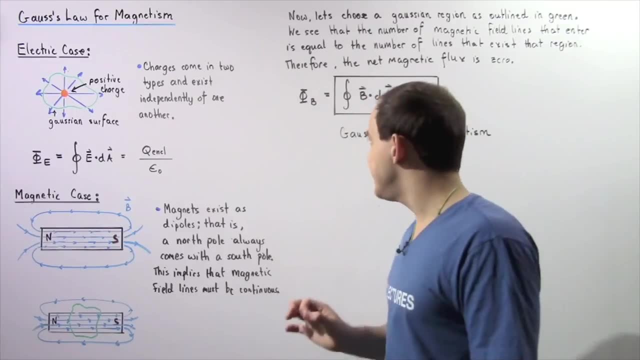 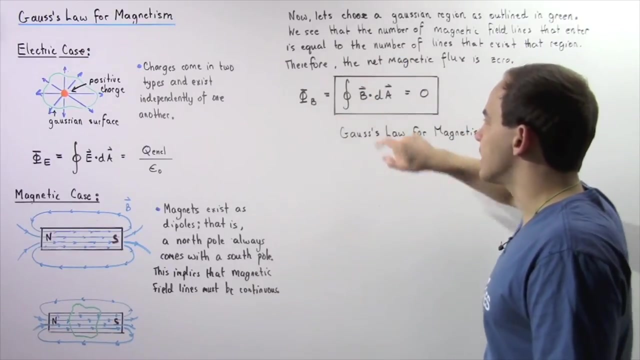 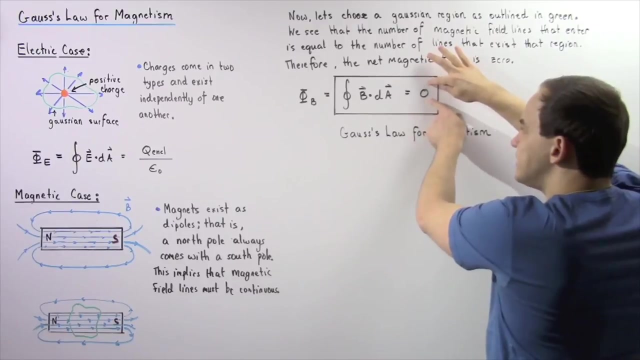 to the number of magnetic field lines exiting the net magnetic flux through the following green Gaussian region is equal to zero. So our net magnetic flux is equal to the closed integral of the dot product of the magnetic field B and our infinitely small area vector dA is equal to.